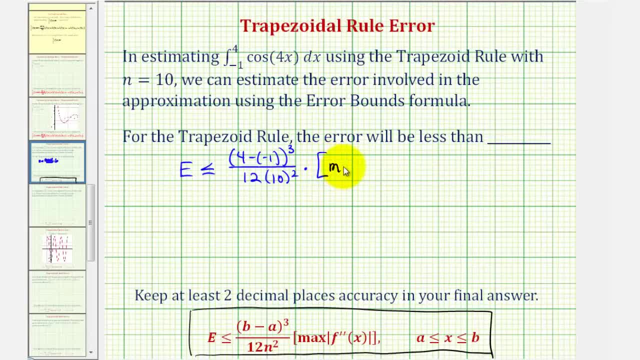 and then times the absolute value of the maximum of the second derivative function on the closed interval from a to b. So we're going to find the second derivative function on the closed interval from negative one to four. So let's go find this maximum function value. 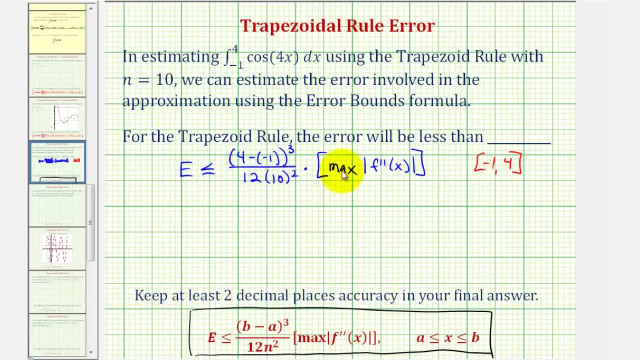 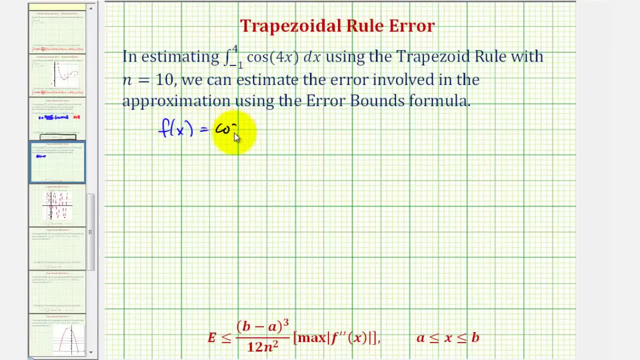 on the next slide and then we'll come back and finish this calculation. So, starting with the integrand function, f of x equals cosine 4x. we want to find the second derivative, so we'll first find the first derivative, which is negative: 4 cosine 4x times 4x. 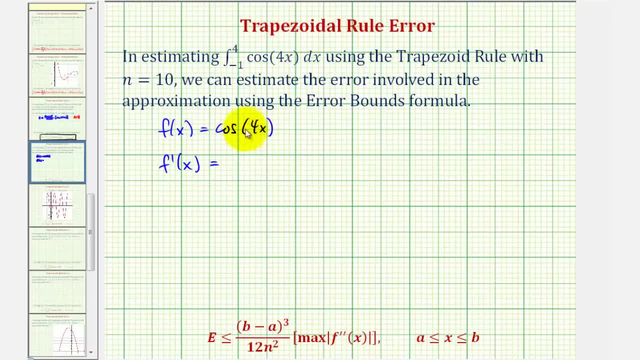 To find the derivative of cosine 4x we have to apply the chain rule, So our derivative will be negative sine 4x times 4, or negative 4 sine 4x. And now the second derivative would be equal to negative 4 times the derivative of sine 4x. 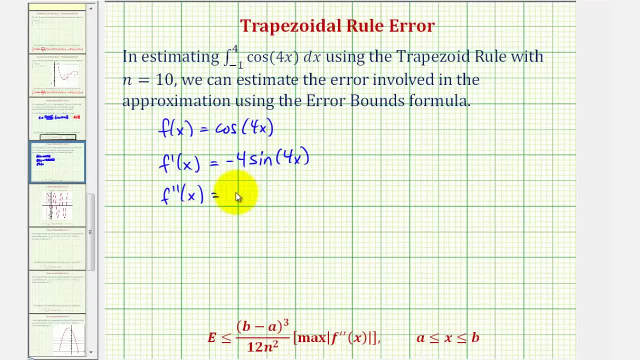 which would be negative 4 cosine 4x times 4, or negative 16 cosine 4x. Now we want to find the maximum function value of our second derivative function on the closed interval from negative one to four. So what we could do is find the derivative of this function. 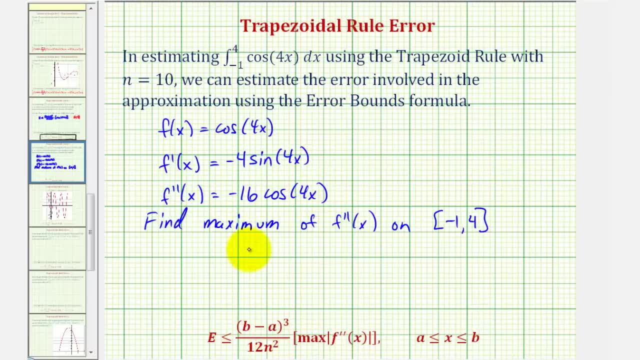 which would be the third derivative, set it equal to zero and solve to find the critical numbers and then evaluate the function of the critical numbers and the endpoints to determine the maximum function value. but in this case we should recognize that the graph of our second derivative function would have an amplitude of 16.. 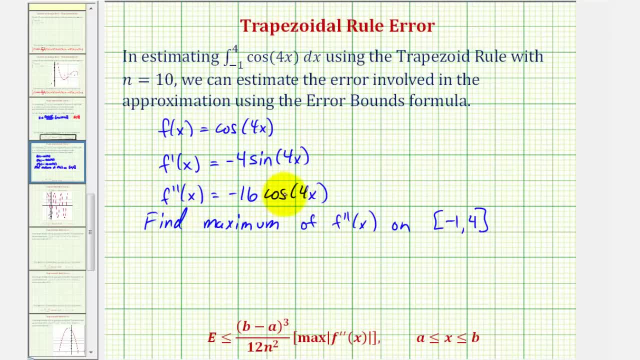 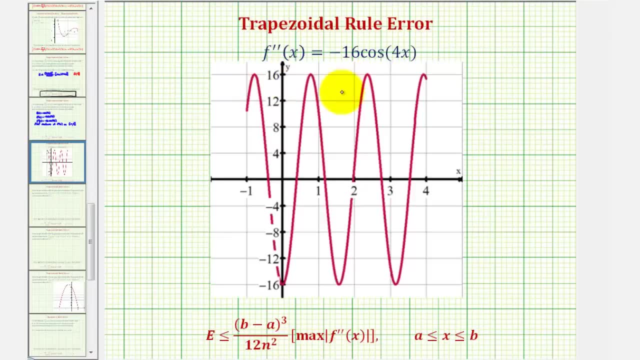 So in this case, let's just analyze the graph of our second derivative function to determine the maximum function value on this closed interval. So here's the graph of our second derivative function And again, because we have an amplitude of 16, we can easily verify the maximum function value. 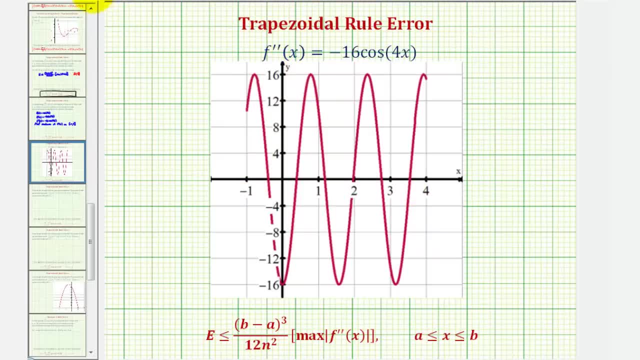 on the closed interval from negative one to four would be positive 16, which actually occurs four times over this interval here, here, here and here. Notice: f of negative one would be some value here, less than 12, and f of four would be some value here, less than 16..